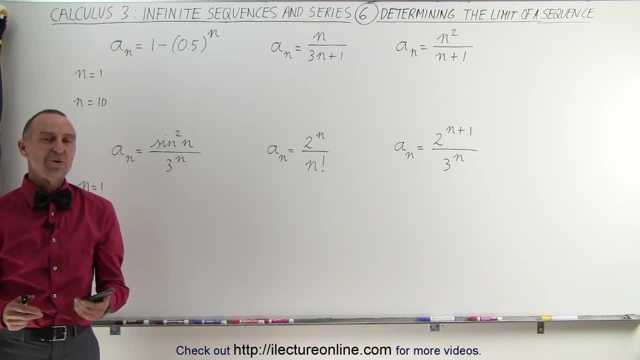 Welcome to ElectronLine. and now let's do a few examples, a few practice examples of finding the limit of a sequence. Now, the same kind of rules apply to this as you've seen before when you're trying to graph algebraic expressions, algebraic functions, where we have numerators and denominators. 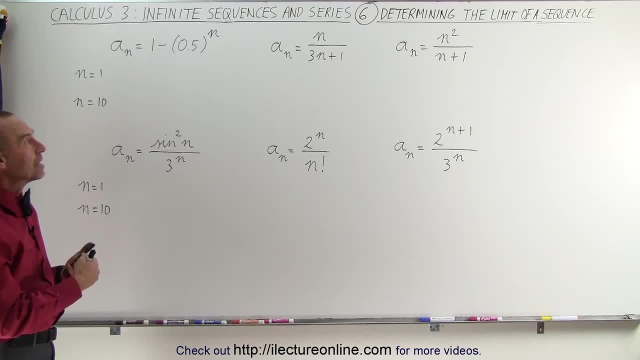 And, of course, as the values get larger, does the ratio of the numerator to the denominator? does it converge to a constant number or to zero, or does it become bigger and bigger and bigger and become infinity? And so that same concept applies here as well. 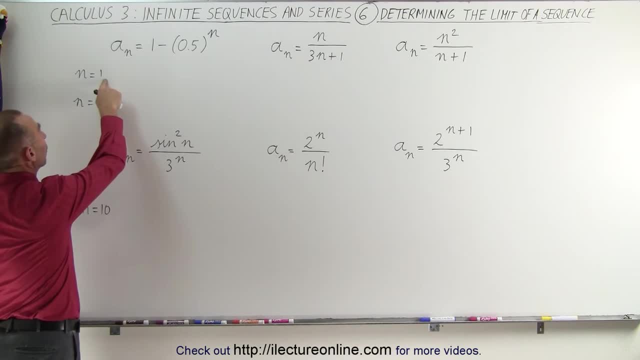 Quite often we can figure it out by simply replacing n by 1 and then doing it again by replacing n by 10, and to see if that number converges to a fixed number or if it gets really big. For example, the sequence: a sub n equals 1.. 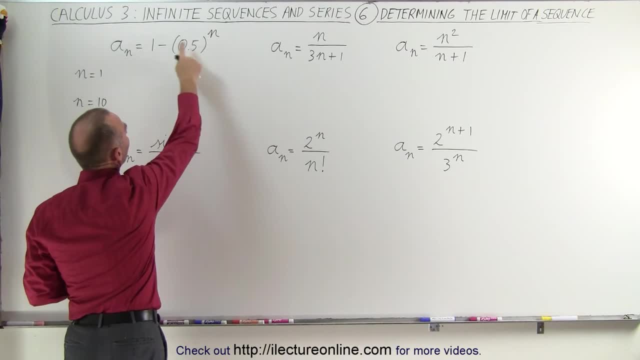 a sub n equals 1 minus 0.5 raised to the n power, We realize that if the number is less than 1 and we raise it to a very big number, this will eventually go to 0, which means in the limit this should become equal to 1.. 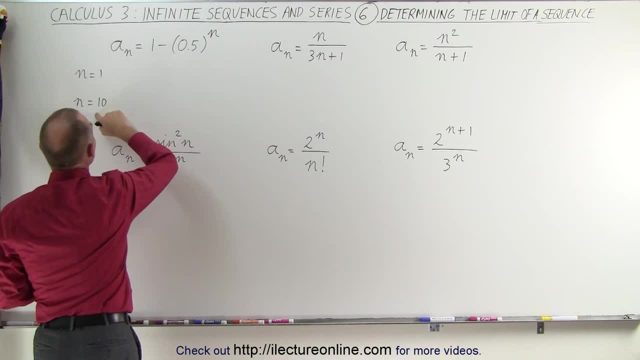 And we can verify that by plugging in n equals 1, and then again for n equals 10, and we'll see what we end up with. So for n equals 1, a sub n becomes equal to 1 minus 0.5, which is 0.5. 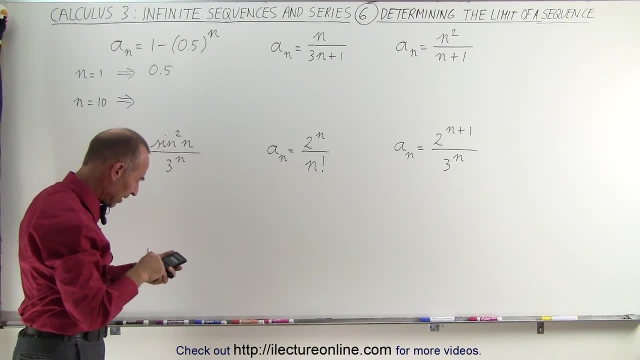 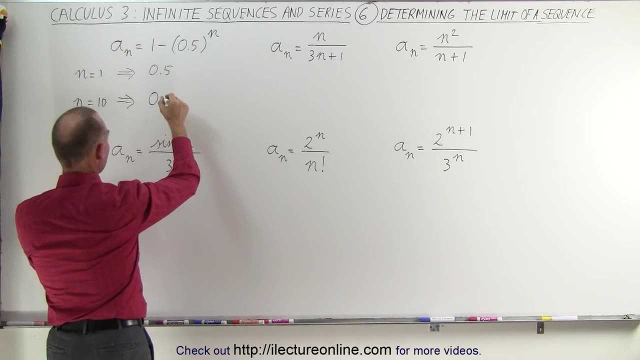 And then when we plug in the value of a sub n, a sub n becomes equal to 0.5.. And then we plug in the value for 10, 0.5 raised to the 10 power. If we subtract that from 1, we get a number which is equal to 0.999. 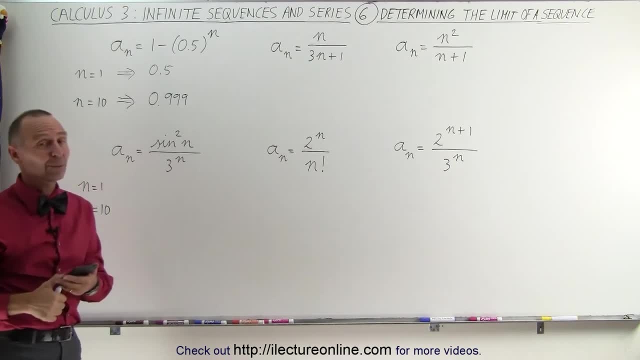 And of course you can see that that approaches the number 1 and we can be fairly sure that as n approaches infinity, a sub n will approach 1.. When we have a situation where we have a fraction and we have an n to the first power in the numerator and n to the first power in the denominator, 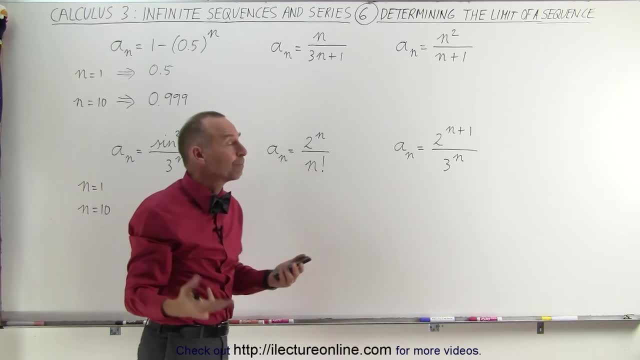 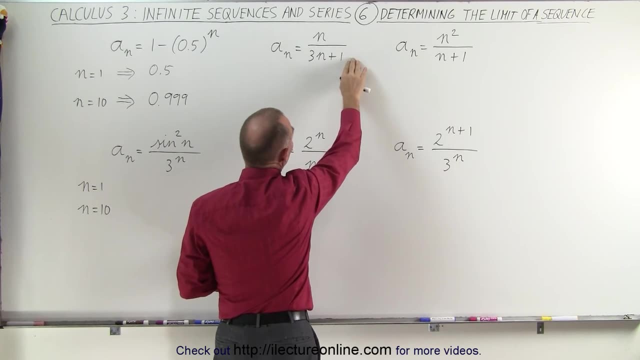 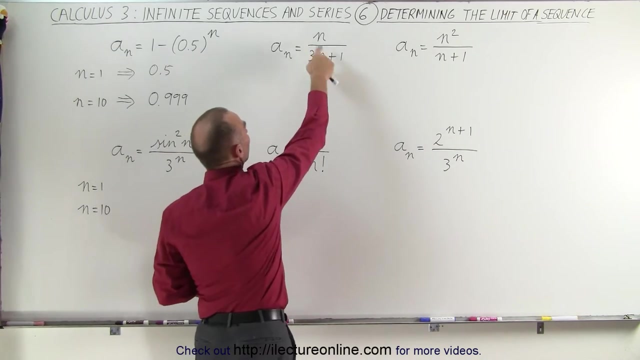 as n becomes really large, this plus 1 becomes insignificant. As the numbers become larger and larger and larger. n divided by n will essentially negate the plus 1 at the denominator. and then we have n divided by 3n, which eventually will converge to 1 divided by 3, as n and n will cancel out. 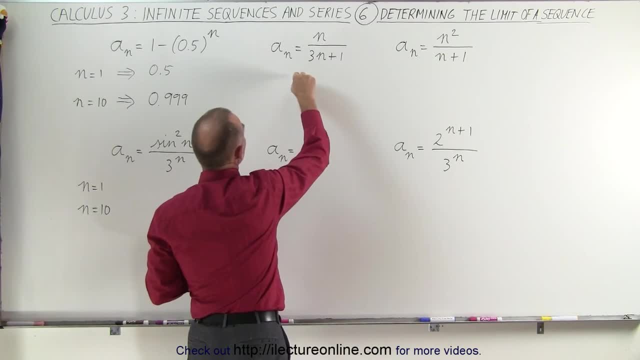 Again, you can see how that happens when you plug in n equals 1.. So for n equals 1, the value will become 1 divided by 3 times 1, which is 3 plus 1, which is 4.. 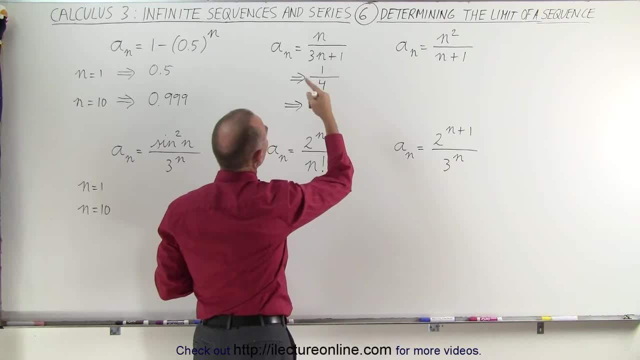 And then, when we plug in the value for 10,, we get 10 divided by 30 plus 1, or 10 divided by 31.. And then we get a value of 0.322, which, in the limit, becomes closer and closer to 1 third. 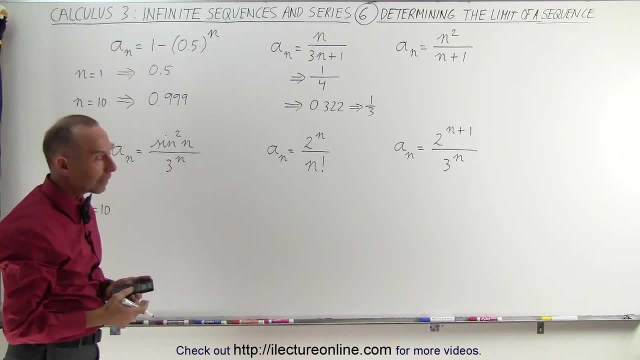 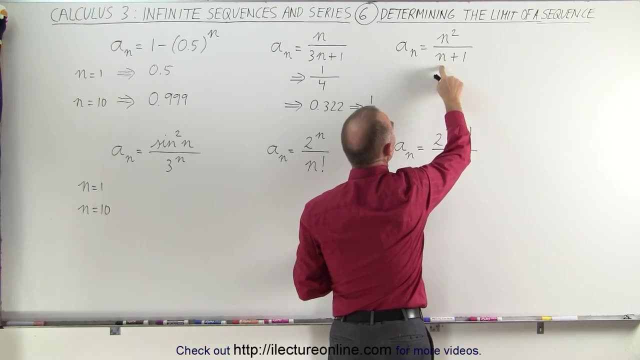 So that would be the limit of that particular sequence. If in this example we have a numerator, we have n to the second power in the denominator, n to the first power If the exponent is larger in the numerator than it is in the denominator. 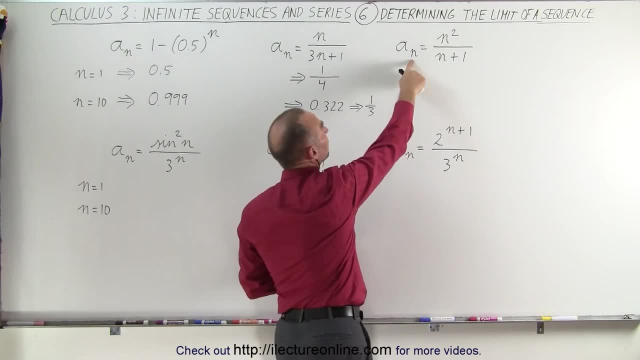 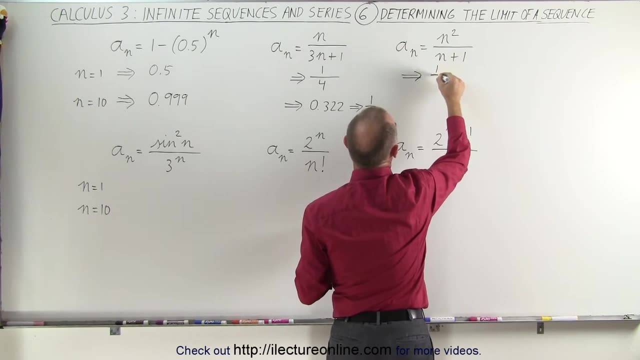 the numerator will grow much, much faster than the denominator as n becomes really big. So in this case you can see: when n becomes equal to 1, that will become 1 divided by 2, or 1 half. But when n becomes equal to 10, 10 squared is 100 divided by 11,. 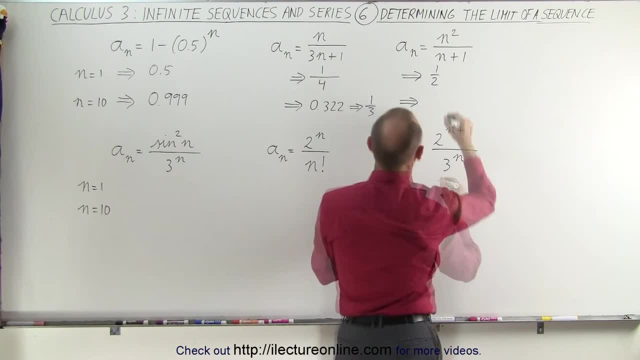 so we have n divided by 11. We get the number 9.09, and as n becomes larger and larger and larger, eventually you see that this will go to infinity, so it does not converge. In this example we have a numerator. 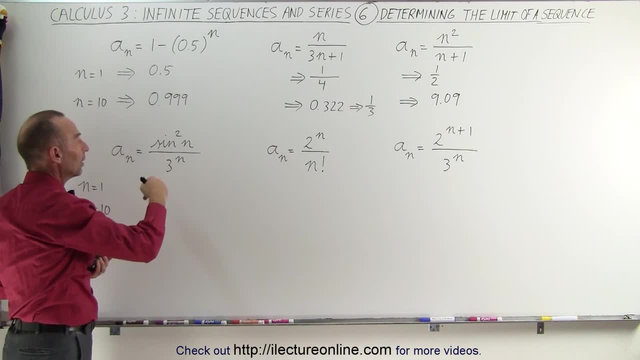 which can only vary between positive 1 and negative 1.. So as n gets larger, this will keep ping-ponging back and forth between positive 1 and negative 1, and since it's squared, it will ping-pong back and forth between 0 and 1.. 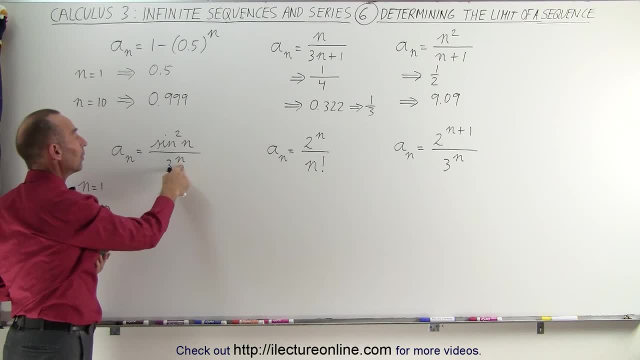 In the denominator we have 3 to the n power. Thus, as n becomes larger, the denominator becomes larger and larger and larger. A number between 0 and 1 divided by a larger and larger number will eventually converge to 0.. 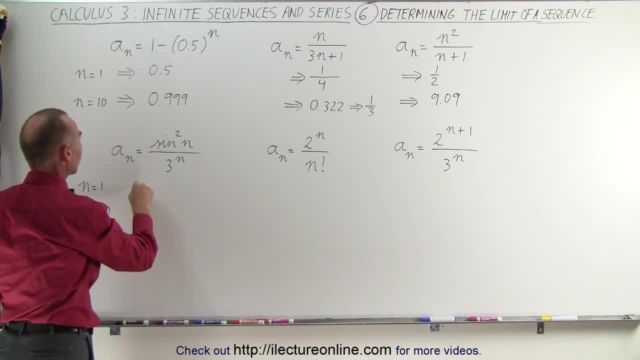 So this will also converge. If you plug in the number n equals 1, let's see here 1, take the sine of that, square that, and then divide that by 3 to the 1,, which is 3,. 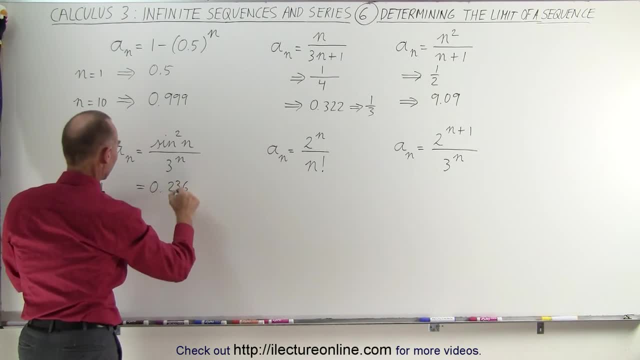 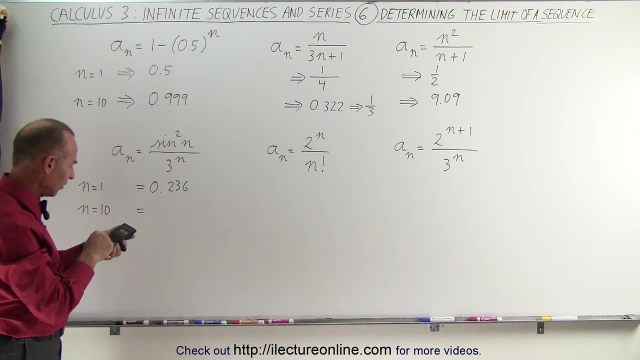 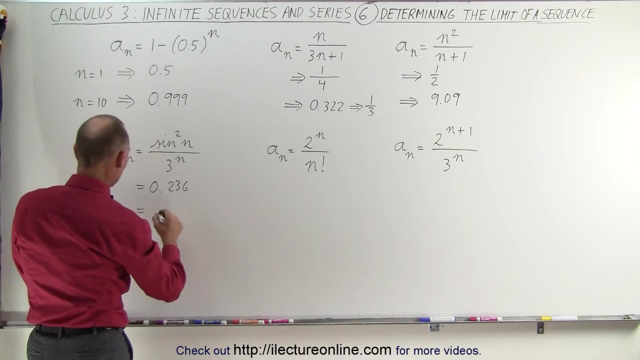 we get 0.236.. Now, when we use the number, n equals 10, so we get n. take the sine of that square, that number, and then divide by 3, raised to the 10 power, and we get, well, a pretty small number. 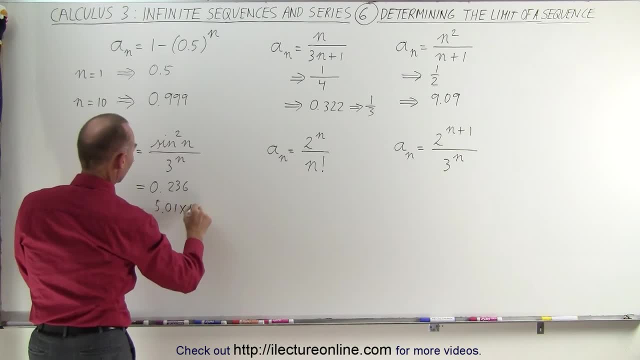 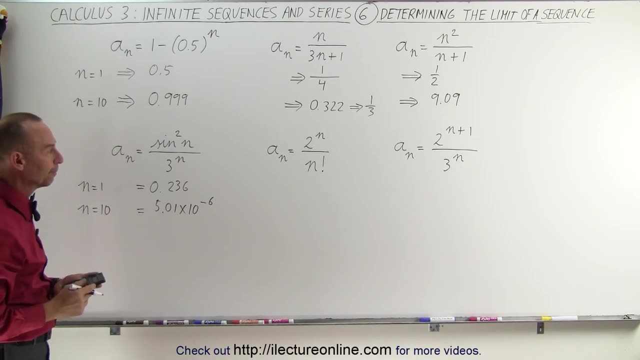 so this becomes 5.01 times 10 to the minus 6, so you can see that this is a very small number. If n continues to grow, this will converge to 0.. The next one is kind of interesting, which is what we're perceiving. 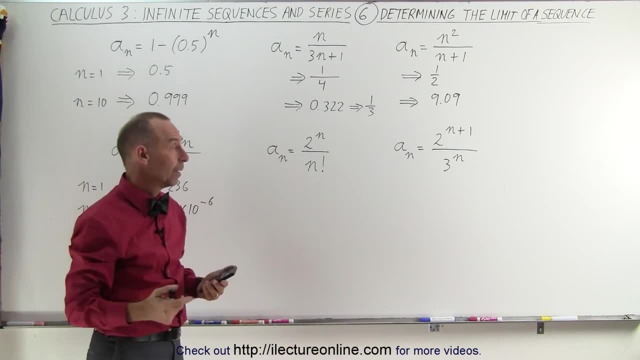 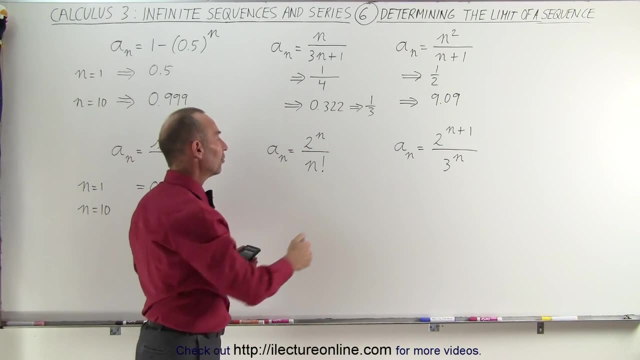 As n becomes very large. 2 to the n will of course become a very large number, But it turns out that n factorial grows faster as n becomes larger than 2 to the n power. So eventually the denominator will become larger than the numerator. 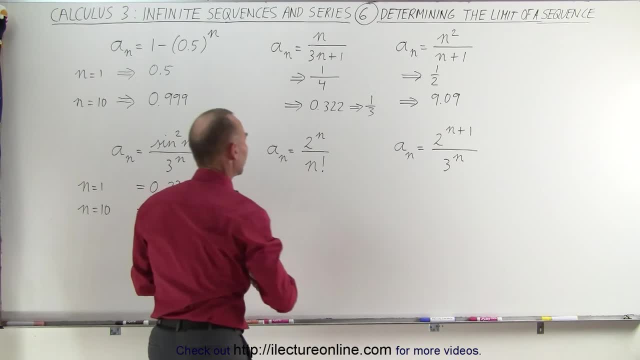 and therefore this will eventually converge to 0.. Well, let's find out: if n is equal to 1,, 2 to the 1, power is 2, divided by n factorial. when n is 1, that will simply be 1.. 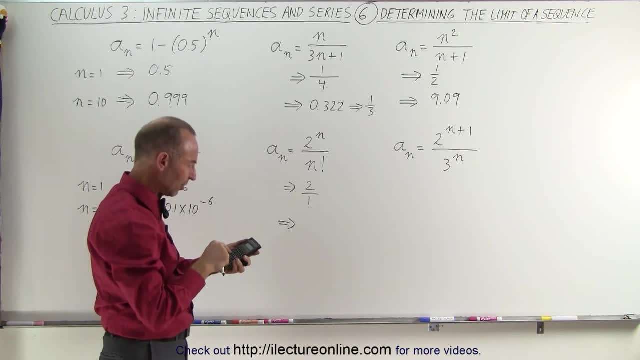 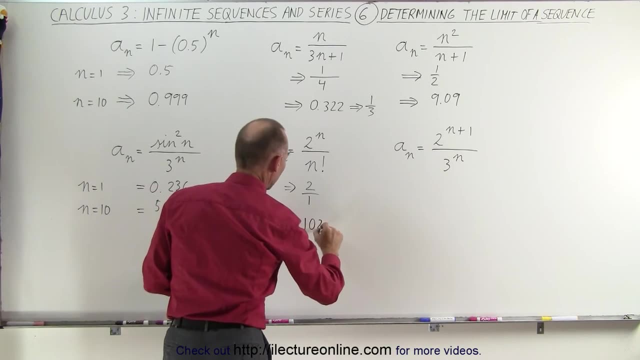 But n becomes 10 to raised to the 10 power, I think it's 1024,. let's find out. Yes, it's 1024, divided by n, factorial. and let's see where's my factorial button. 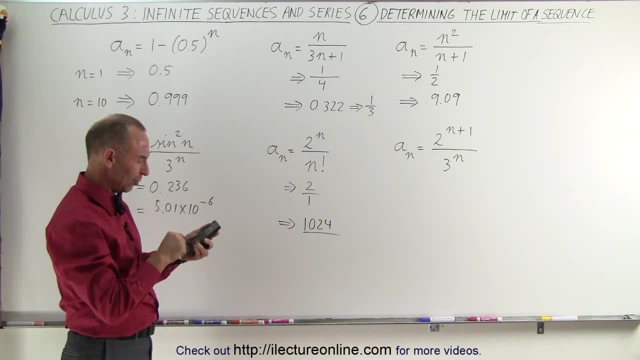 Well, I don't know where my factorial button is, but I'll quickly go. 1 times, 2 times, 3 times, 8 times, 9 times 10 equals and yes, that's a really big number. so that would be equal to 3.7 billion. 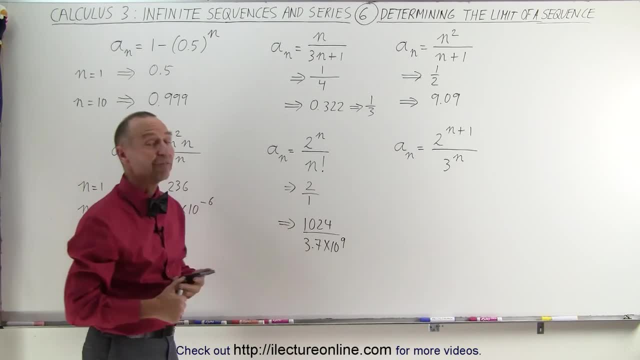 3.7 times 10 to the 9 power. so you can see that very quickly, as n gets large, n factorial becomes a huge number and this number will be closer and closer and closer to 0.. And finally, we have this right here. 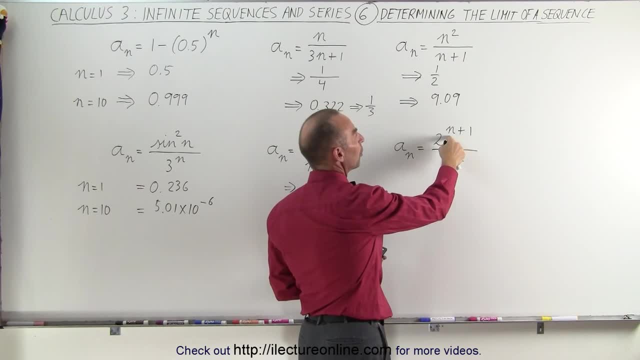 2 to the n plus 1, divided by 3 to the n, Even though the exponent in the numerator will always be larger than the exponent in the denominator. but the base is a 2 here and it's a 3 there. 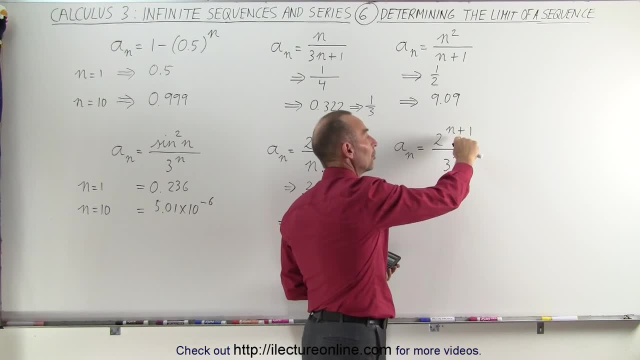 And eventually there only will be one difference between one unit difference between n plus 1 and n, and since the base here is smaller than it is there, the denominator will actually begin to grow faster. Let's check and see if that's the case. 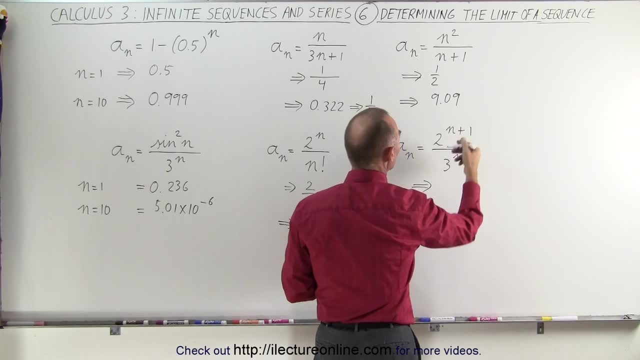 When n is equal to 1,, 2 to the 1 plus 1,, that's 2 to the second power, which is 4, divided by 3 to the 1 power, which is 3.. But if n is equal to 10,,